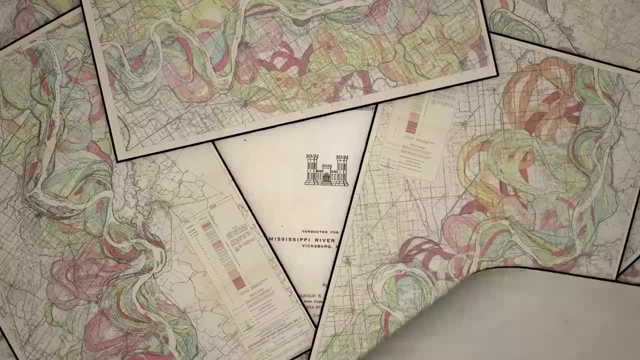 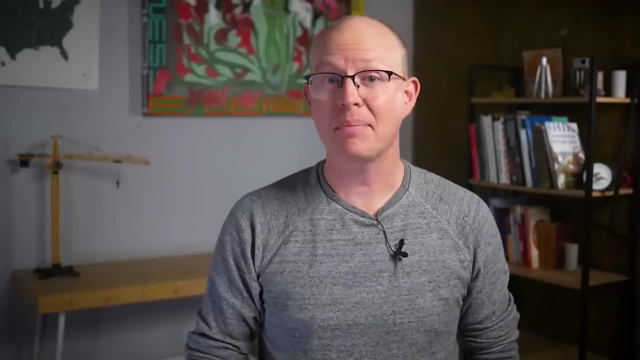 not just the 1944 path of the Mississippi, but of all the historical paths it's cut through the landscape over thousands of years. Although astonishing to see on a map, that meandering path represents a major challenge, not just for the people who live and work near the river. 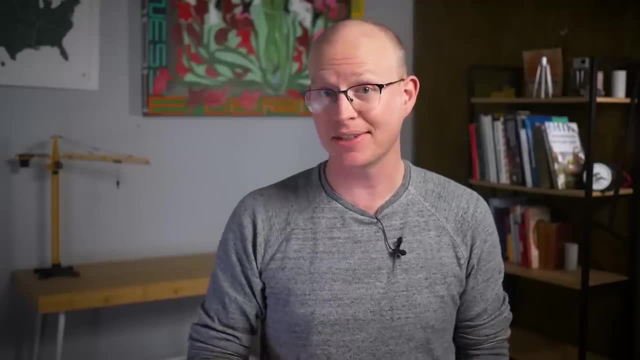 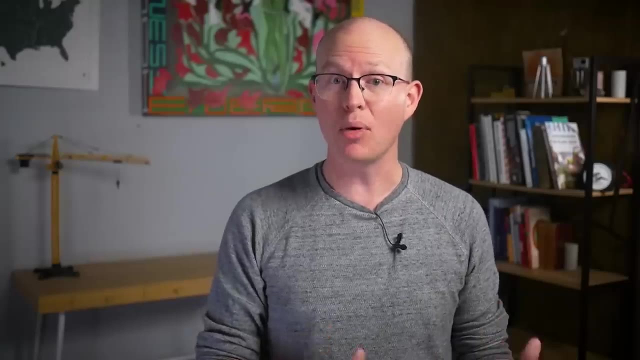 but the people around the world who depend on the goods and services that it supports, And that's a lot of people. What the Native Americans called the Father of Waters is one of the most important freight corridors in the entire United States And a huge proportion of 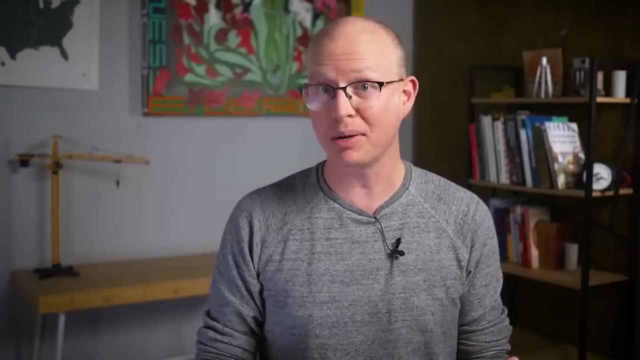 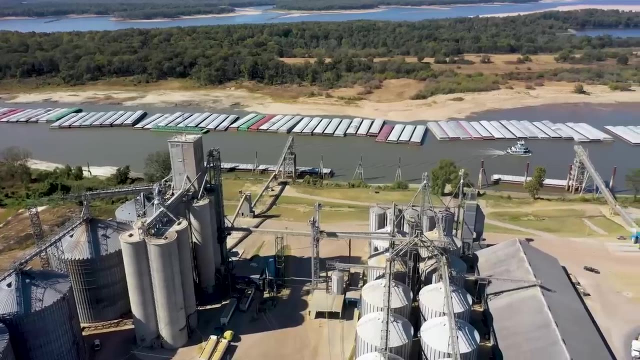 the grains we export to other countries is transported on barges along the Mississippi River. A change in the river's course could bottleneck freight traffic, cripple the economy and potentially even result in a global food crisis. In the 80 or so years since Harold Fisk's report. 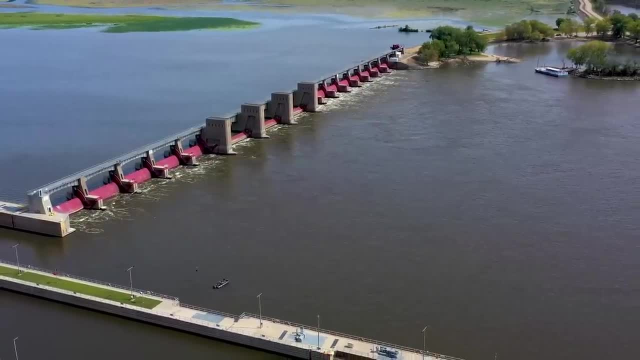 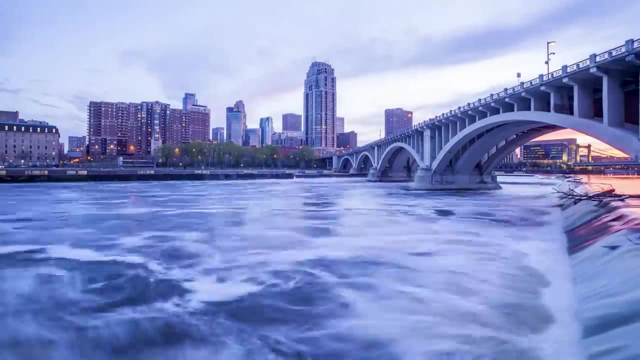 was written. we've spent billions of dollars on infrastructure just to coerce the mighty Mississippi to stay within its current channel. And that's only a single case study in a battle that's happening non-stop around the world between human activity on Earth and the dynamic nature. 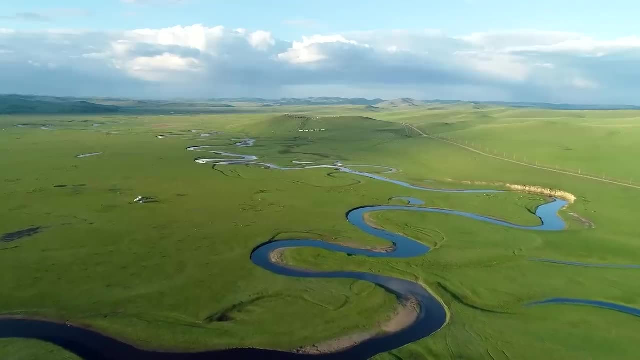 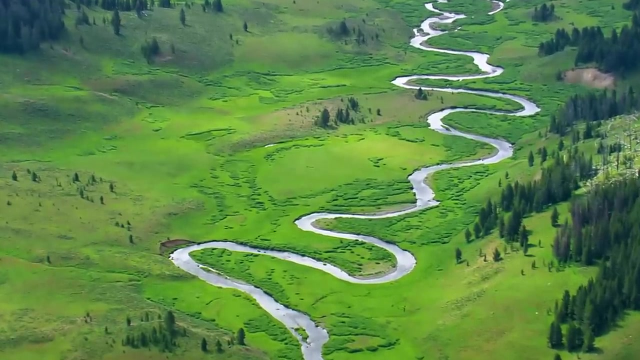 of the river, And that's the reason why we're still here, Even though the natural shifting and meandering of rivers and streams can seriously threaten our infrastructure, our economy and even the environment. it's not something that many people pay attention to or even know about at all, Because the timescale is slow. 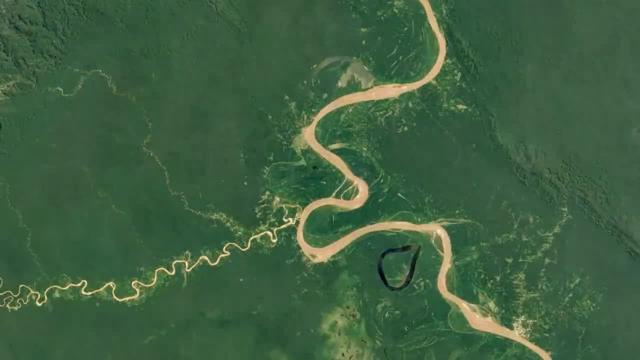 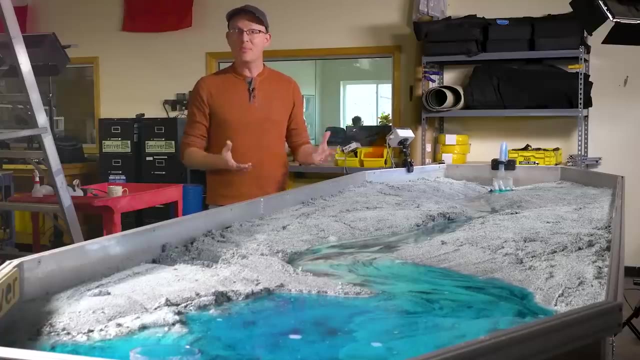 and gradual- you don't see it in headlines- until it becomes a serious problem, And the factors that affect how rivers move don't really follow our intuitions. So we've teamed up with ImRiver, a company that makes physical river models, called stream tables, to. 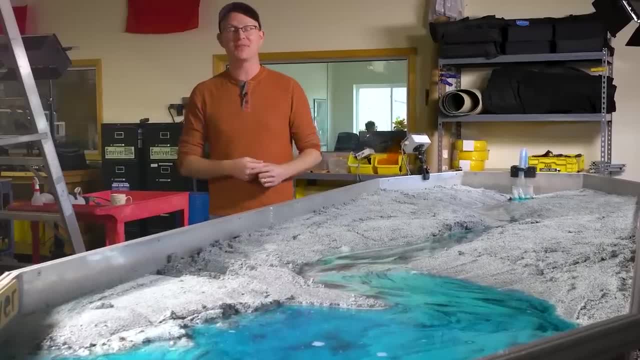 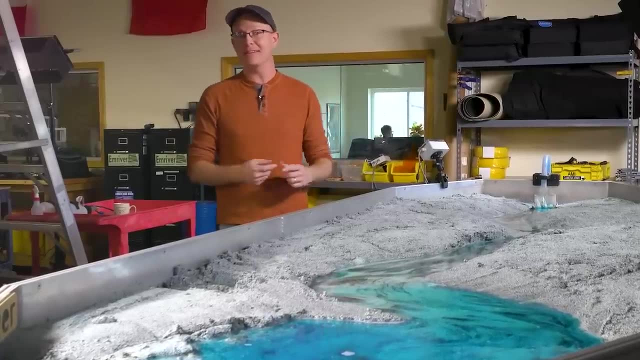 create a two-part series on the science of why rivers shift and meander and the tools that engineers use to control that process. We're here on location at their facility in Carbondale, Illinois, and I'm so excited to show you these models. I'm Grady and this is Practical Engineering In today's episode. 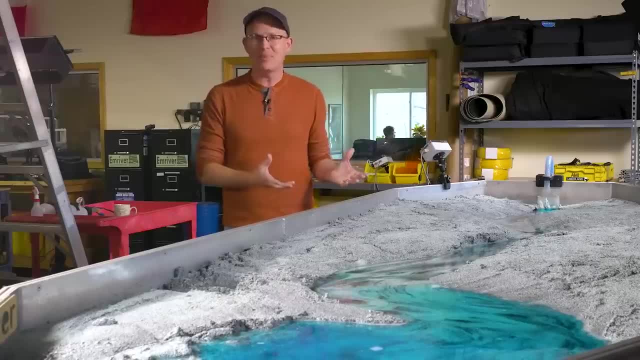 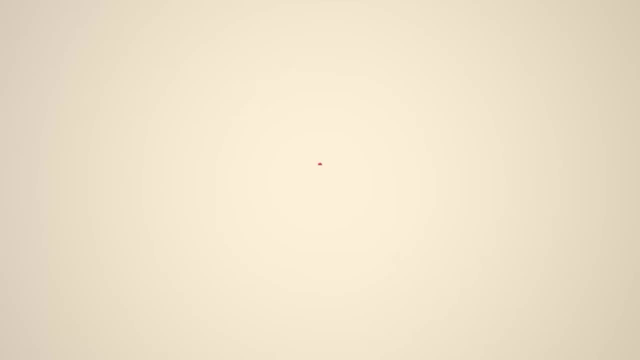 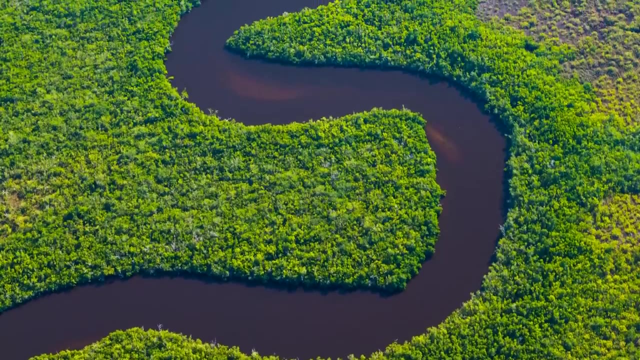 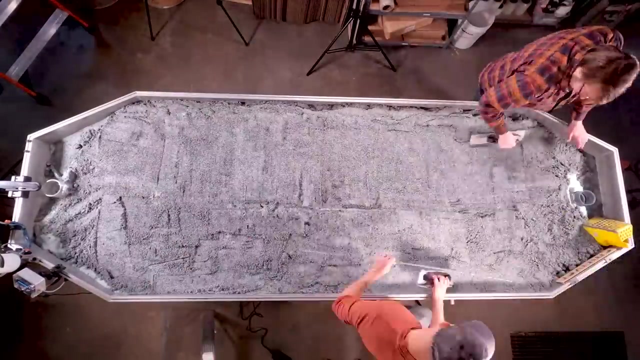 we're talking about fluvial geomorphology or the science behind the shape of rivers. If someone asked you to engineer a channel for water to flow between two locations, what path would you choose? Probably a straight line between them, right? It's the simplest. 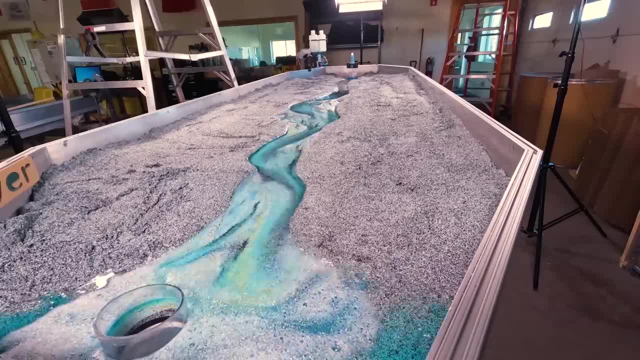 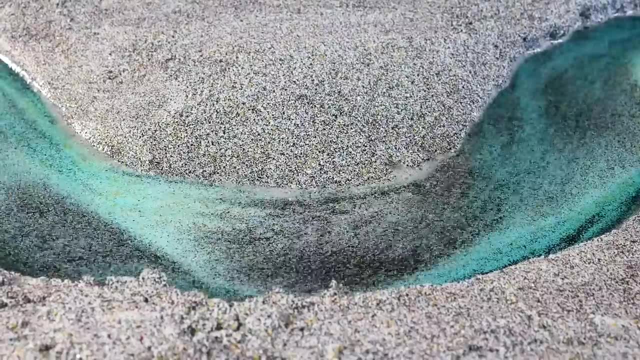 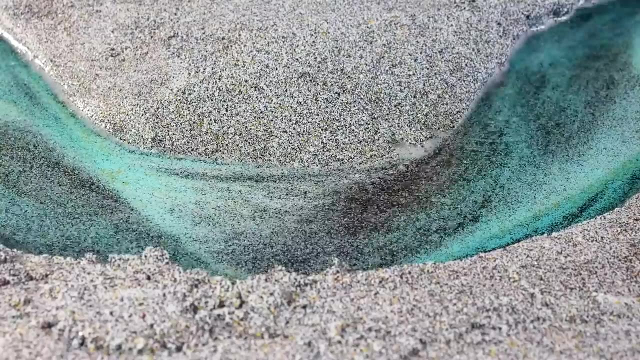 and most cost-effective choice, so why doesn't Mother Nature choose it? This river table is full of media that represents earthen materials like silt, sand and gravel. Each particle size has a different color To make it easier to differentiate, and the online video compression algorithms love this stuff. 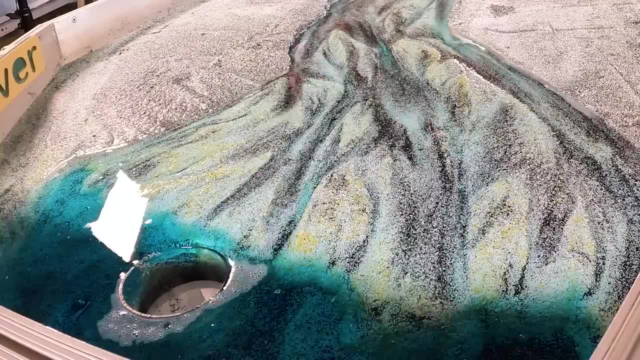 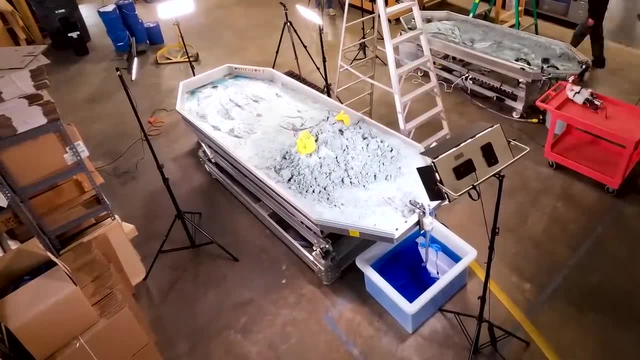 Water flows in at the top of the table and out at the bottom, so we can witness the actual physical processes that happen in real rivers. In the real world, this river system would be tens or hundreds of miles long, and what happens in this model over the course of a few hours? 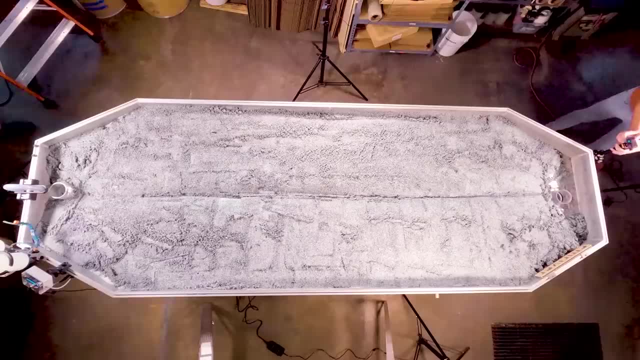 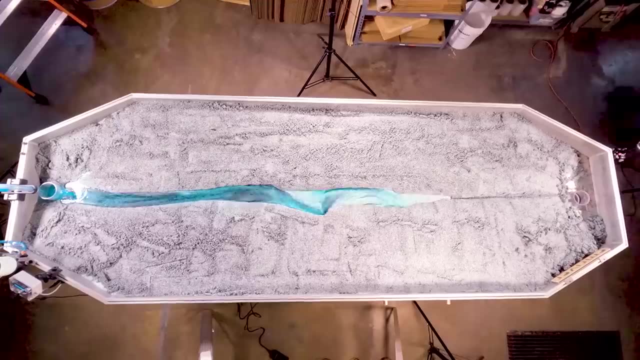 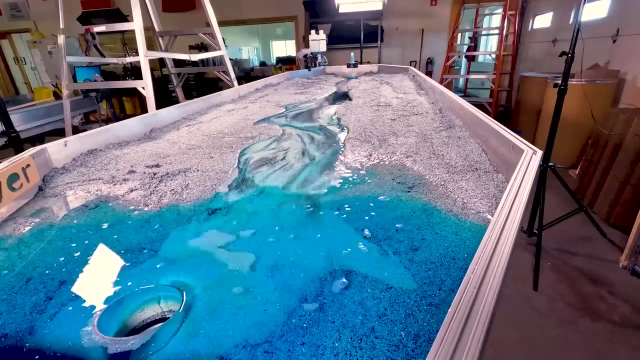 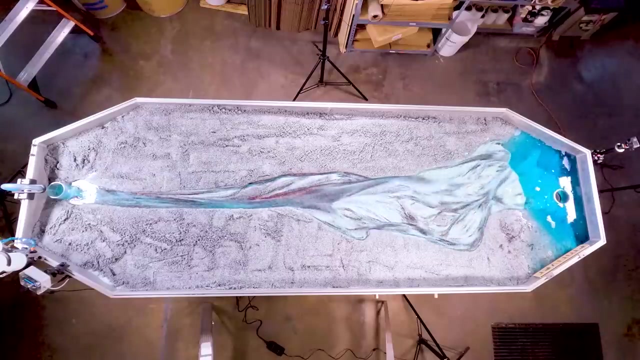 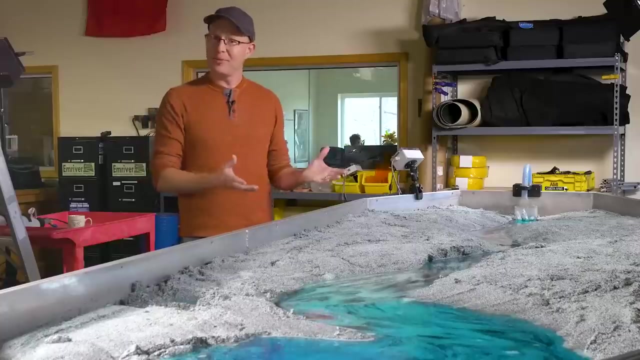 might take hundreds or thousands of years as well. Let's create that straight path in the earth connecting the inlet and outlet of the stream. table, set the water flowing through it and just see what happens. Did the river behave the way you expected, or was the formation of the meandering path? 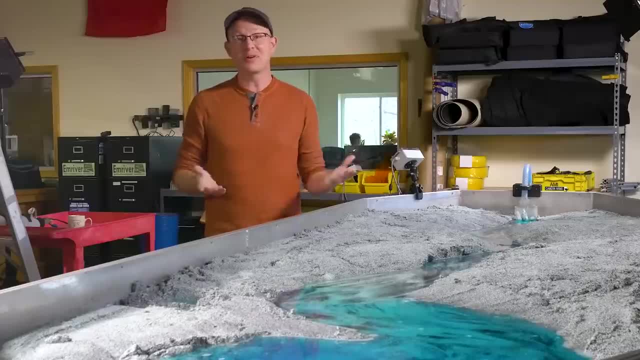 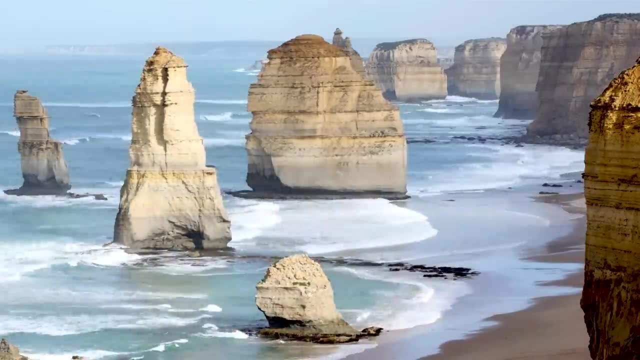 a little bit unintuitive. Hopefully, by the end of this video it will make perfect sense. We learn about the process of erosion even when we're really young. Wind and water carve at the earth, transporting the material from one location to another. 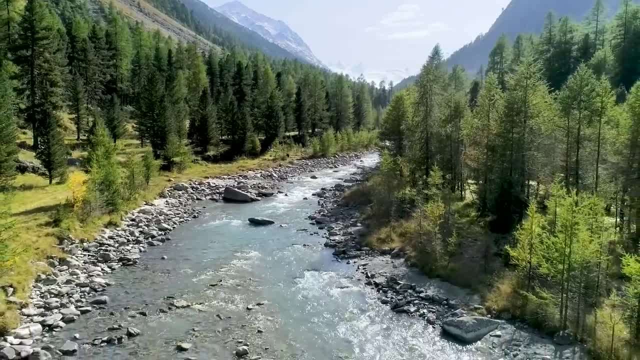 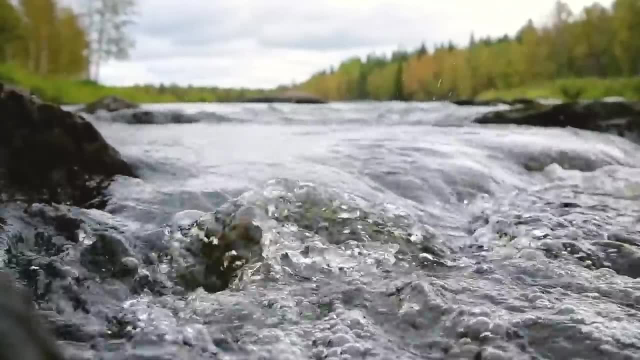 In most places, erosion happens so slowly that you could never watch it in action, like growing grass or drying paint. But take a look at a river and you immediately see erosion underway. All you have to do is dip below the surface of the water and look. We usually think: 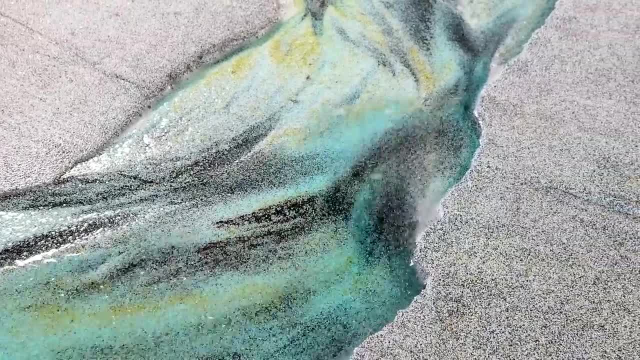 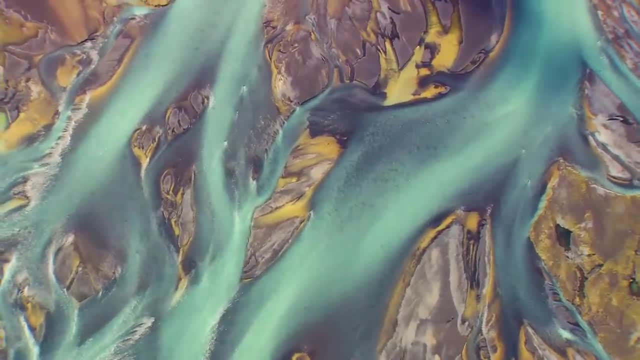 of rivers as highways for water, but they also transport another material in enormous quantities: sediment. All that silt, sand, gravel and rock that erodes from the earth, cascades and concentrates in rivers and streams, where it's carried through valleys and eventually. 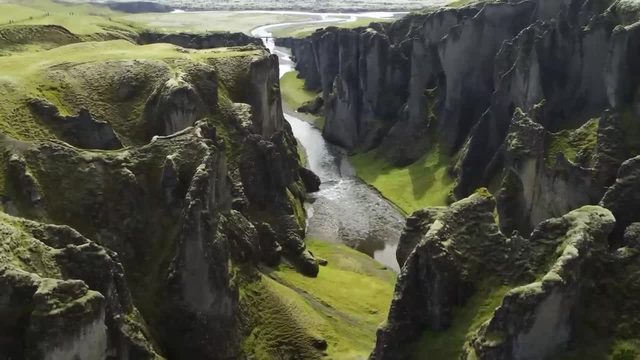 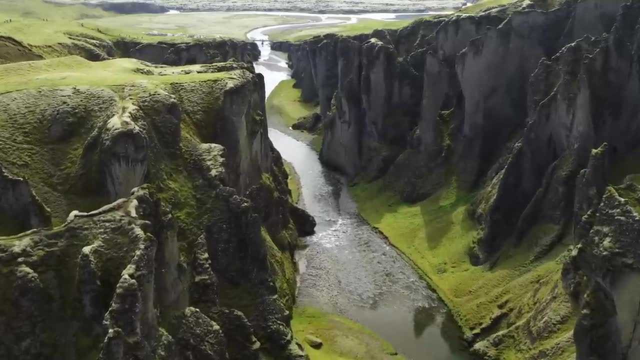 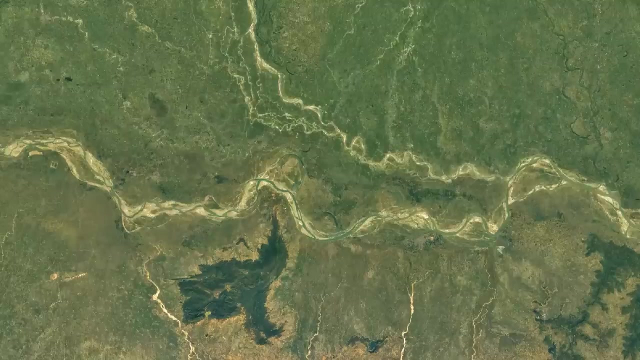 out to lakes and oceans Because of their power to move rock and soil. the shape of earth's landscape, the geomorphology, is hugely influenced by river systems, Maybe because the processes themselves happen so slowly. it took a long time for science to develop around how and why rivers 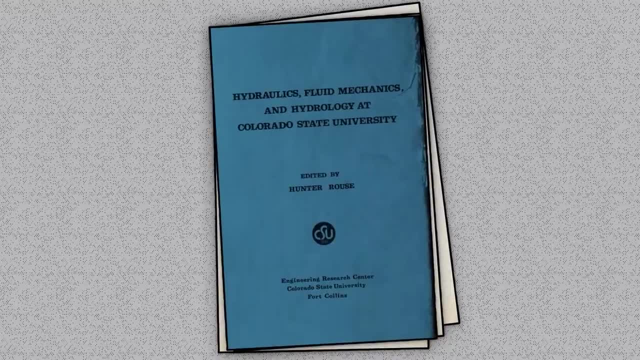 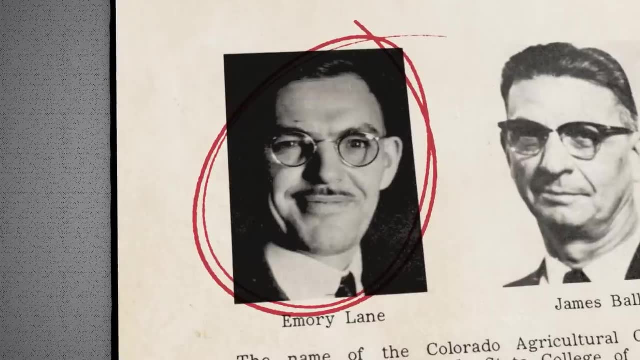 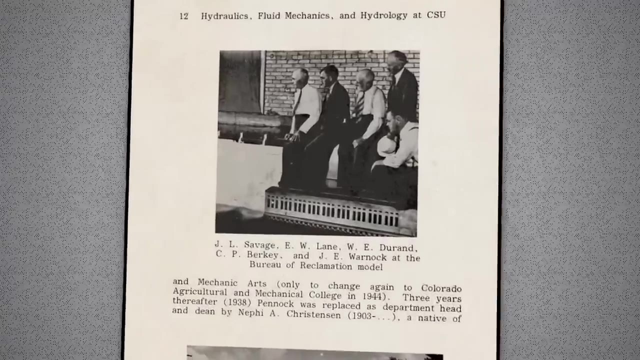 change their paths through the landscape. But in the 1950s a civil engineer and hydrologist by the name of Emery Lane quit his job at the US Bureau of Reclamation to serve as a professor at Colorado State University. Through his time at the Bureau, he worked in hydraulic laboratories. 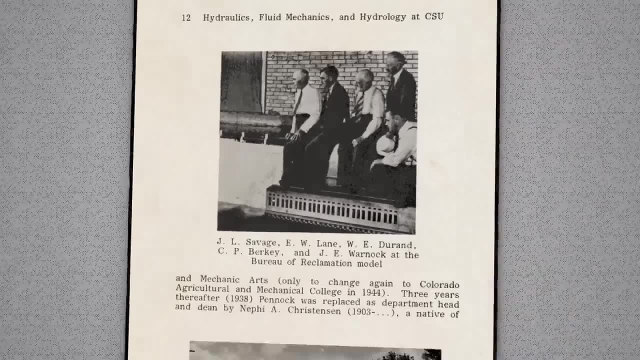 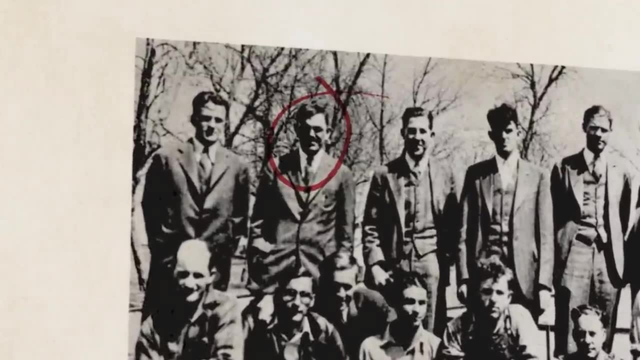 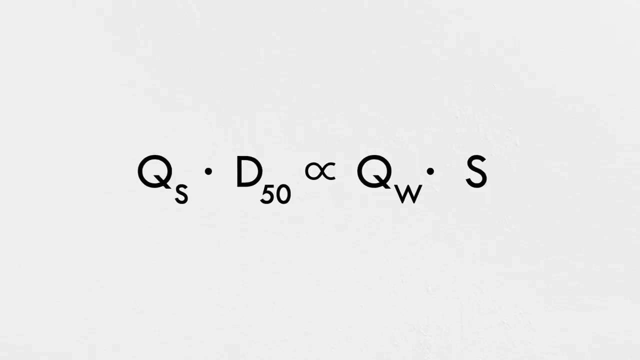 studying the interactions between water, soil and rock. By the time he accepted his appointment, he was well on the way to developing a unified theory of sediment transport. In 1955, he published his landmark equation that's still used today by engineers, geologists and other professionals in 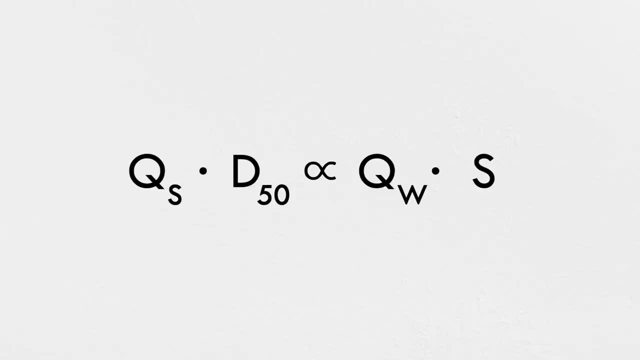 the river sciences And, just like a lot of the most famous equations in history, it doesn't look too complicated. It says that in a stable stream, the flow of water multiplied by the slope of that stream is proportional to the flow of sediment in the stream multiplied by the size of that. 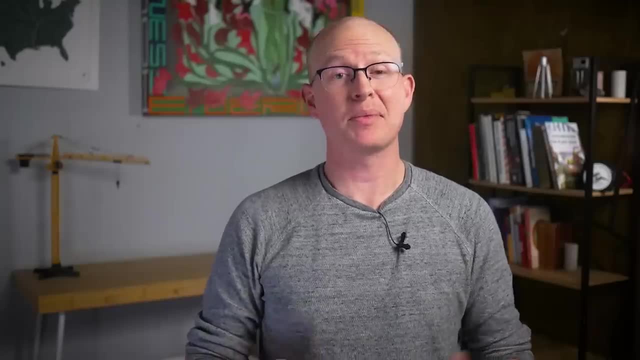 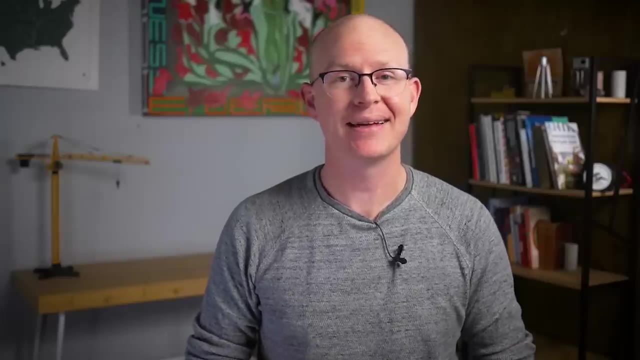 sediment. It seems simple, just four parameters. But you know it's also a funny looking equation with zero context. so maybe you're not feeling like an expert just yet, But with the help of the stream table I can show you the beauty of this relationship and how simple it makes. 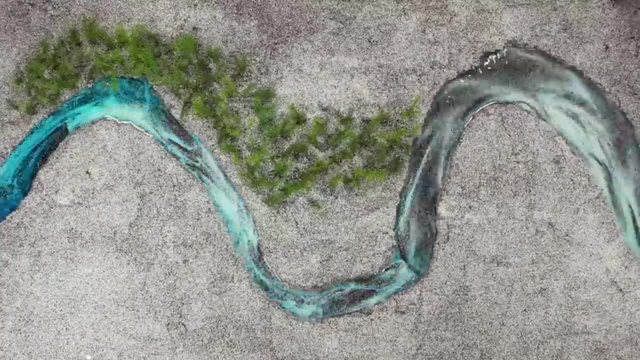 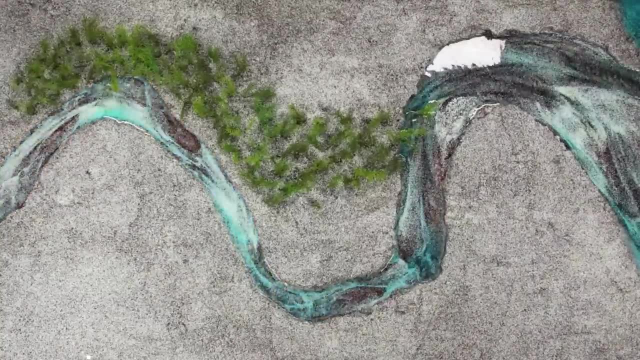 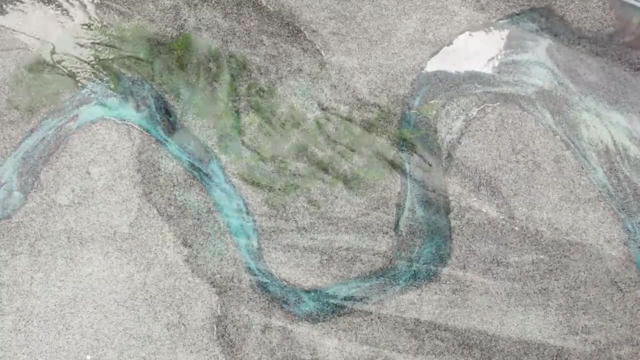 predictions about how rivers will behave. Let's just look at some examples. Say that a large area is hit by a wildfire that burns all the trees and vegetation. Where before you had a lush and verdant landscape with plants, bushes and trees to stabilize the soil, now it's. 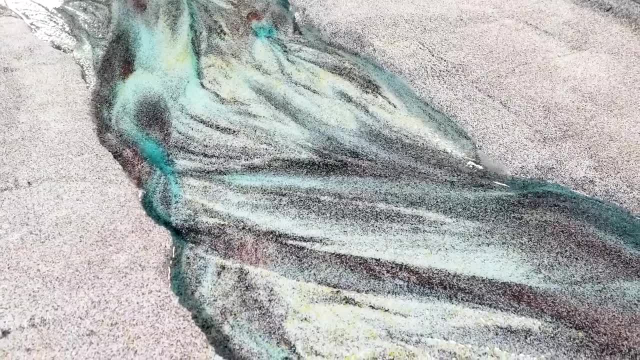 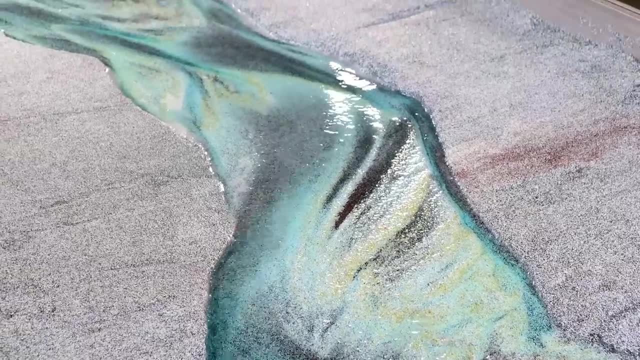 a bare earth When it rains, the water that runs off the burned area erodes the unprotected landscape, washing more sediment into the river than it would have before the fire. We can demonstrate this by simply adding media to the upstream part of the stream table. Can you predict? 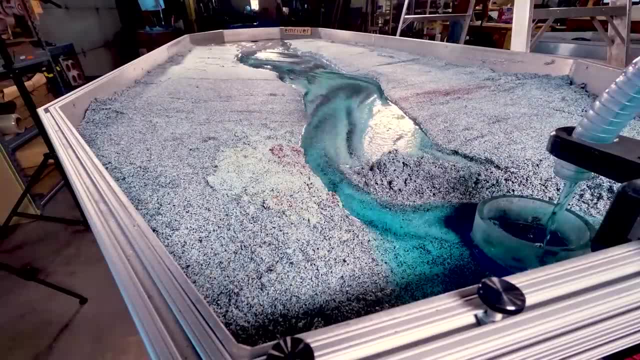 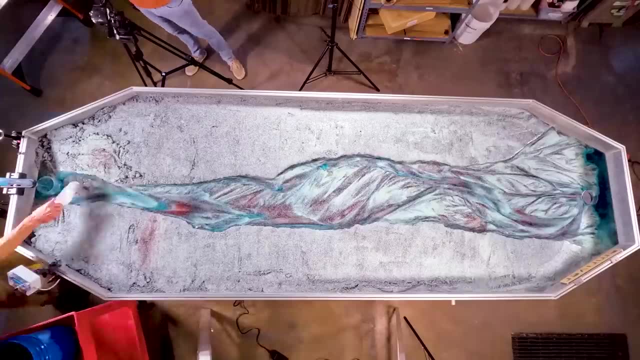 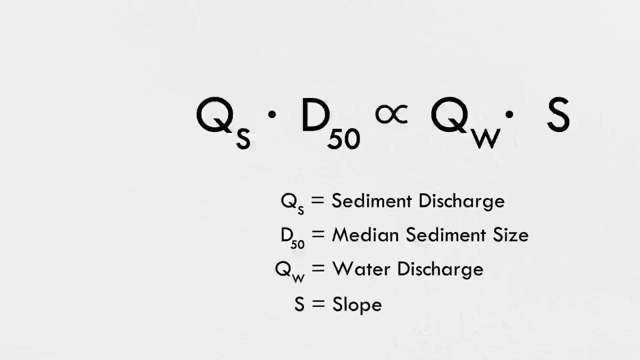 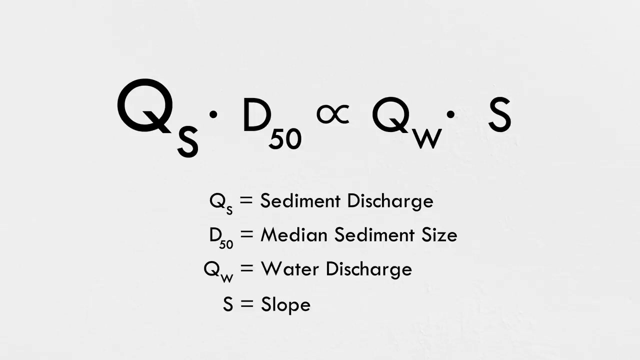 how the river will respond. Let's look back at Lane's equation. We've increased the flow of sediment in the river, but we haven't changed any of the other variables. We didn't change the size of the sediment, we didn't change the flow in the river and we didn't change its slope. That means the two sides. 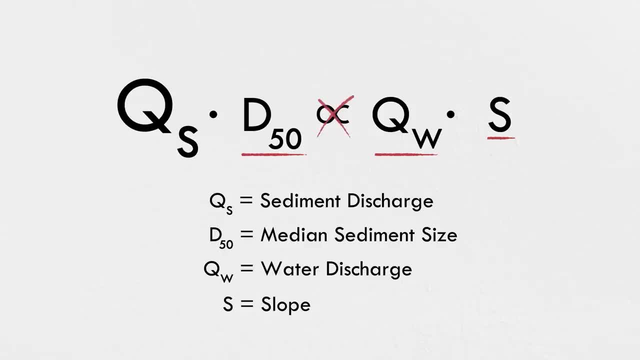 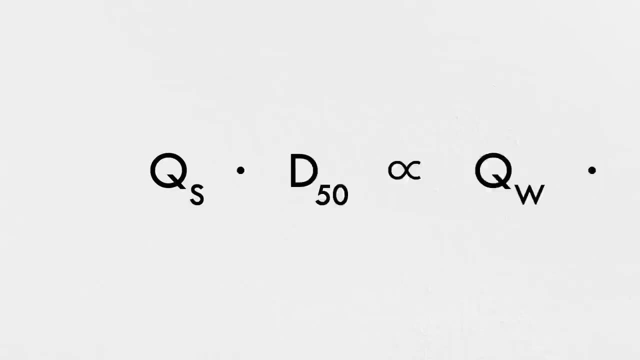 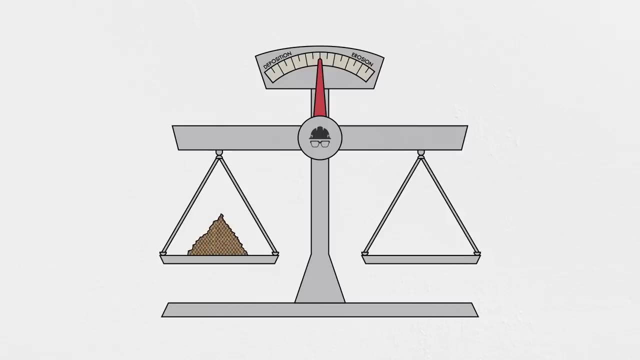 are imbalanced, Lane's equation no longer holds true and the river is out of equilibrium. In other words, this is no longer a stable channel. In fact, we can convert Lane's equation into a diagram to make this much simpler to understand. On one side of this balance is the sediment load. 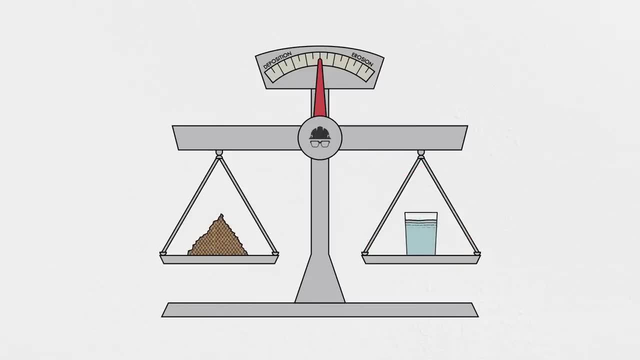 and on the other side is the volume of flow in the stream. Add more flow and you can transport more sediment. Reduce the flow of water and you reduce the flow of sediment accordingly. Pretty straightforward, right? But we still have to include the other two parameters. 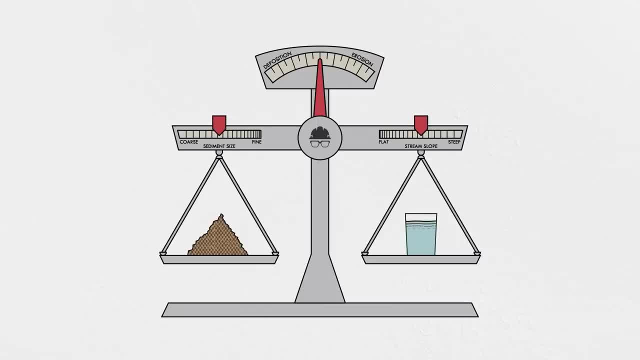 sediment size and stream slope. Now you can see how things get a little more complicated to keep in balance. Any disturbance to any of these four parameters causes the flow of sediment to increase and the flow of sediment to decrease. Any disturbance to any of 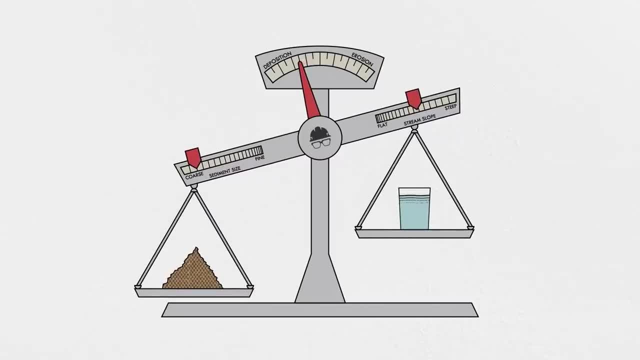 these four parameters causes the flow of sediment to increase and the flow of sediment to decrease, scale to get out of balance, affecting the stream's equilibrium. When that happens, you have short-term consequences and long-term ones too, For the wildfire example, where we 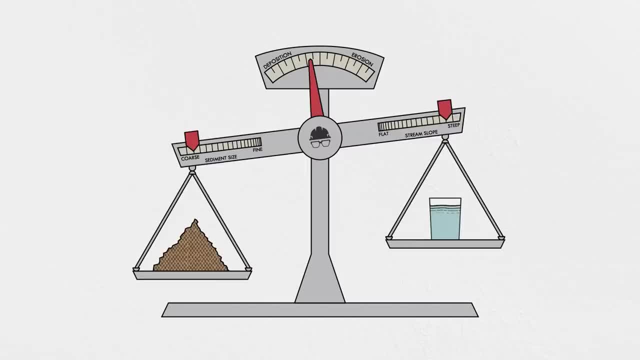 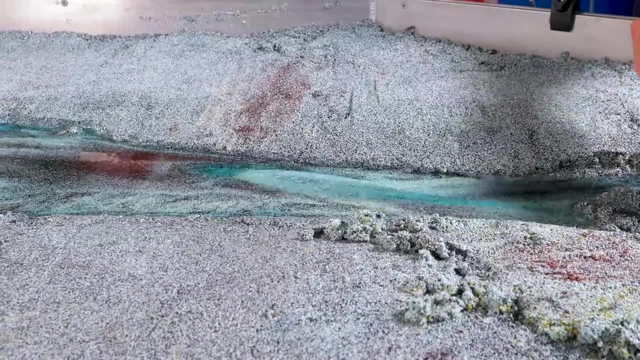 increase the sediment load in the stream. the top of the balance swings left toward deposition. There's not enough water to keep the sediment in suspension, so it's going to deposit within the bed of the river, like we're seeing here in the model. The flow in this example just 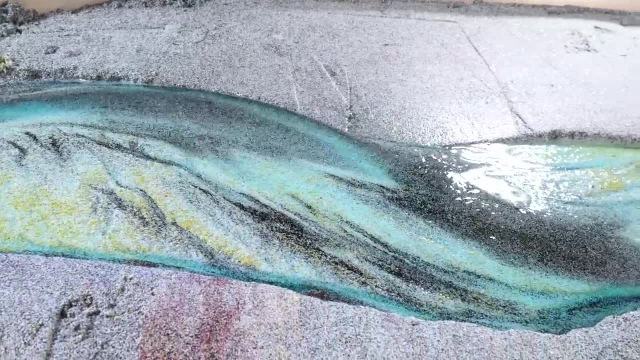 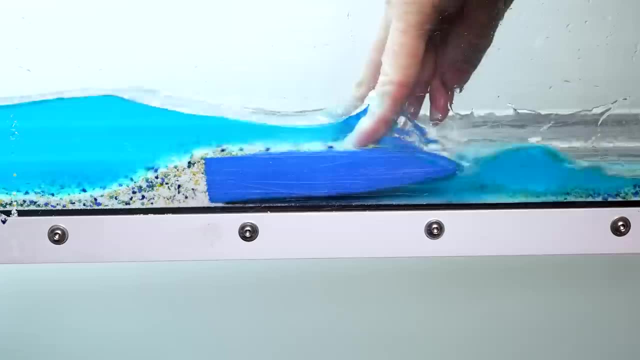 can't hold all the sediment we're washing into it, so it accumulates in the bed and banks of the channel over time. Here's another example of a natural disruption to a river system that's easier to demonstrate in the flume, Beavers build a small dam across the channel. 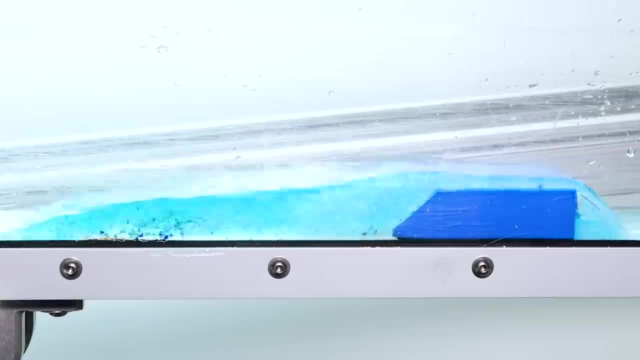 creating a pond that slows down the flow. As the velocity of the stream reduces, heavier sediment settles out. That means the water below the beaver dam only carries the fine particles of silt and clay. downstream You can see the lighter white particles being. 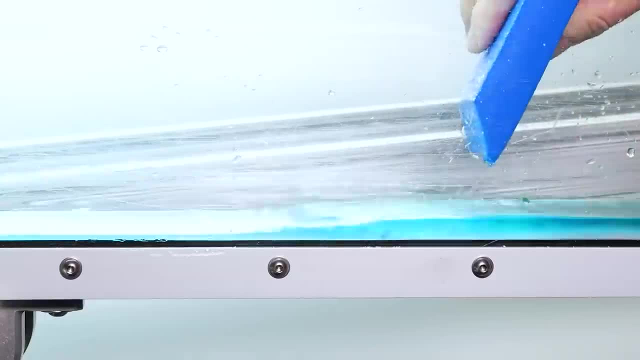 carried away, while the darker, heavier ones get caught behind the dam. Let's take a look at another example of a natural disruption to a river system. that is easier to demonstrate in the flume. look at Lane's balance to predict what will happen to the stream When we reduce. 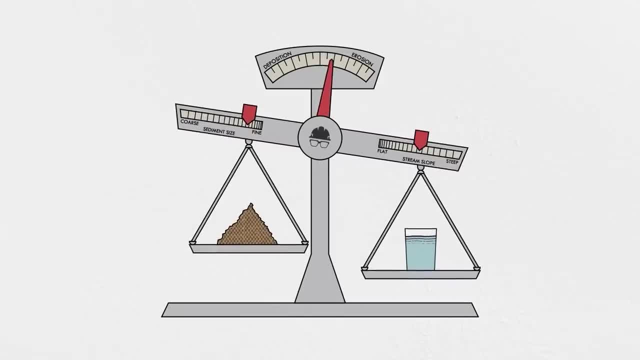 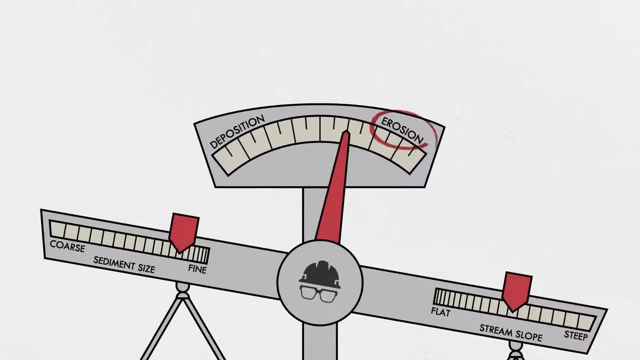 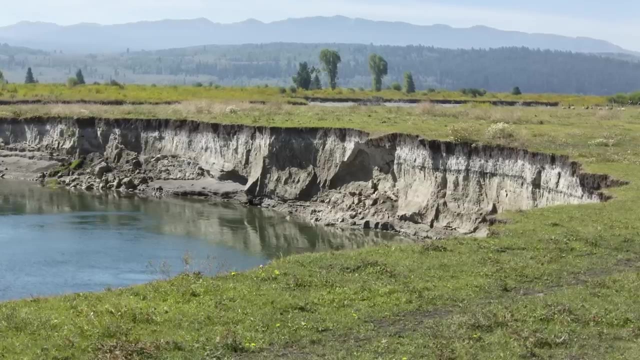 the size of the sediment load in the river. it shifts the left side of the balance inward and again we lose our equilibrium. But this time, instead of deposition, we can expect the stream to erode downstream, And downstream of a dam, human or beaver made is a common place to find erosion occurring. Let's 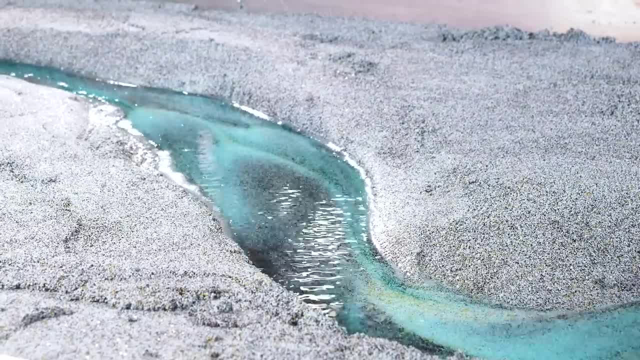 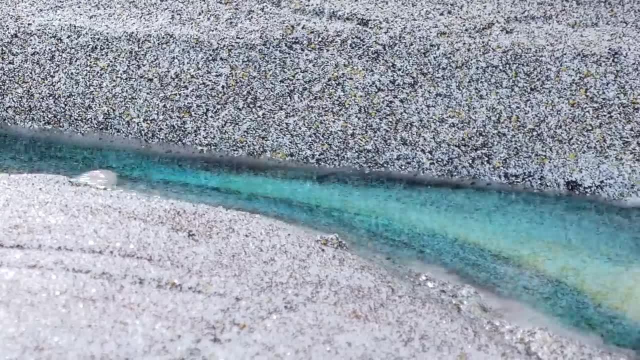 look at one more example of a natural disturbance to a river: changes in the flow. After all, rivers rarely carry a constant volume of water. Their flows change with the seasons and the weather with tremendous variability. That includes floods, where heavy precipitation within a watershed. 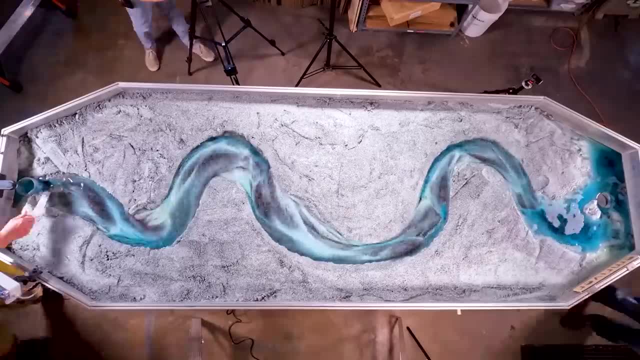 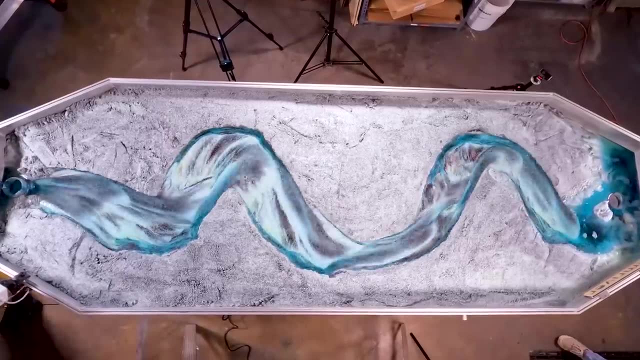 converges toward valleys to swell the rivers and streams. We can simulate a flood in our model channel just by turning up the flow And hopefully at least this parameter matches your intuitions. You can easily see the sediment being carried downstream by the increased flow of water. The banks of the 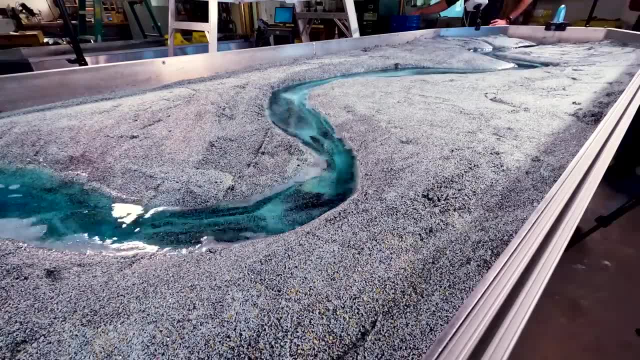 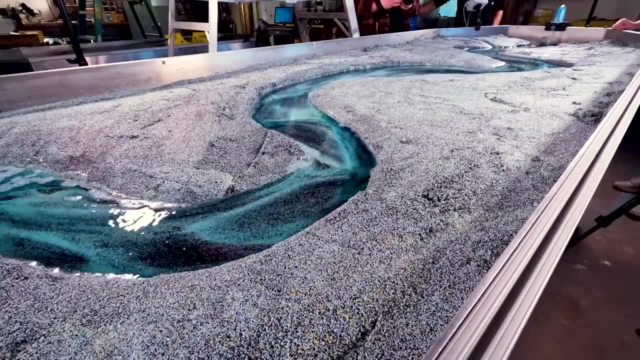 river are not as dense as they used to be in the past, but they are still eroding and the material is carried away by the flood. Looking at our diagram, it's easy to see why, If we increase the flow of water, the 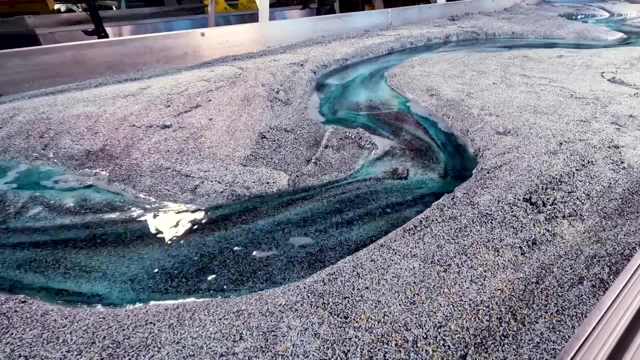 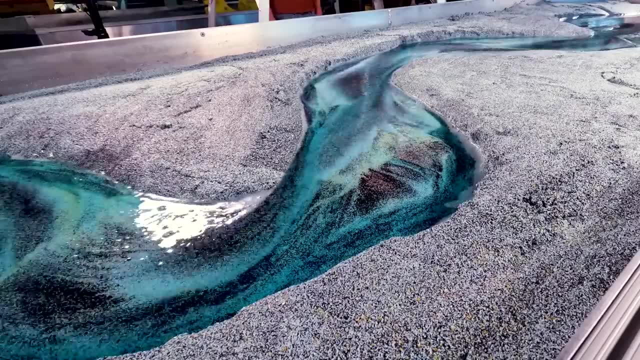 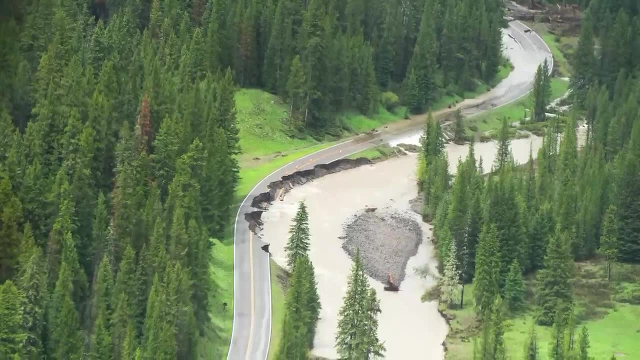 scales out of balance, leading to erosion of the channel. These disturbances to a channel's equilibrium seem relatively benign and even beautiful in the stream table, but they can represent a serious threat to property, infrastructure and even the environment. Erosion causes rivers to shift, washing away roads. 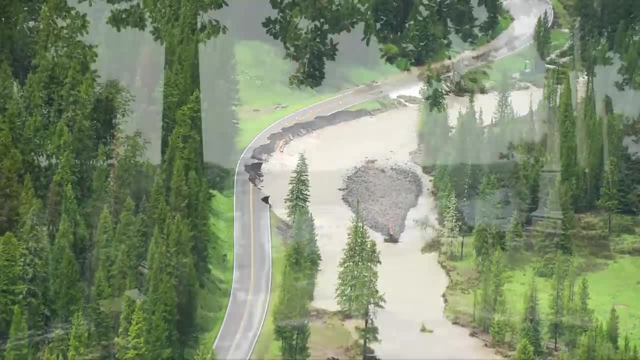 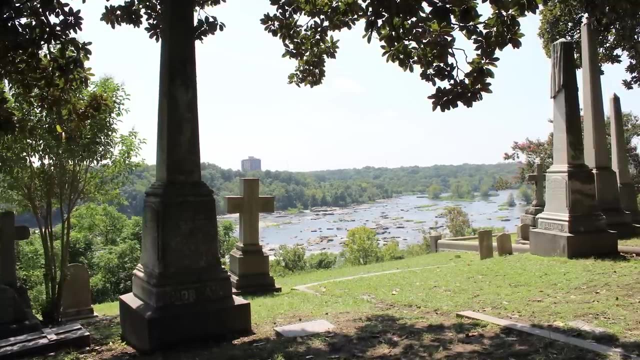 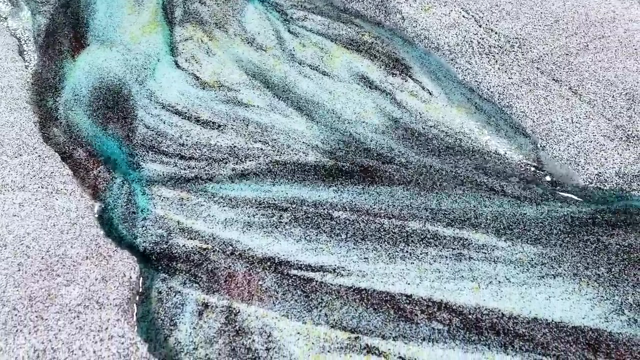 underground utilities and even destabilizing structures. I worked on a project once with a river running alongside a cemetery. Imagine the haunting headlines that a little erosion could create. On the other hand, deposition in a river channel can also create serious issues. Sediment can choke a navigation. 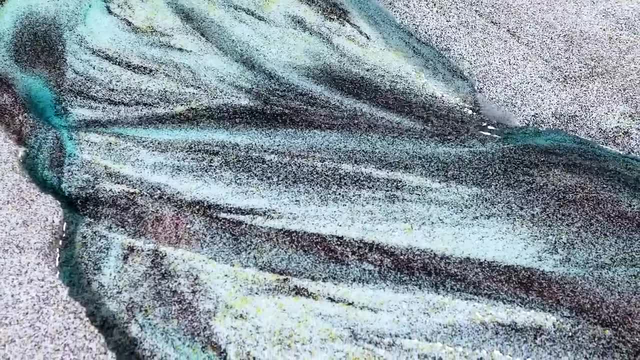 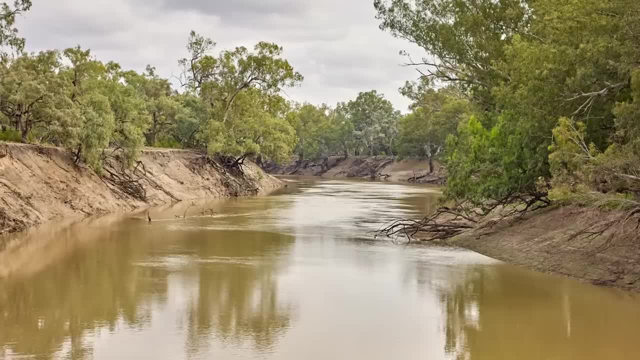 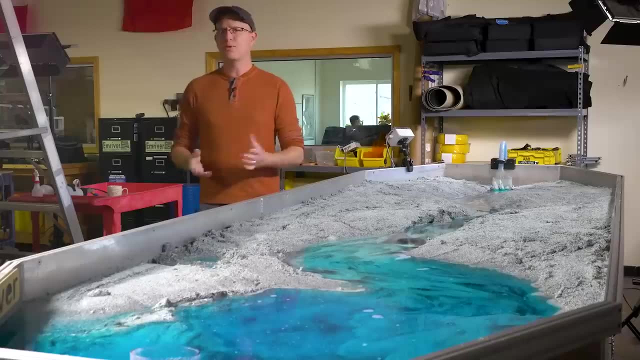 channel, reducing its capacity for freight traffic, and fill up reservoirs, reducing their storage volume. It can damage the habitat of native fish and other wildlife, and deposition can reduce the ability of a river channel to carry water, increasing the impacts and inundation during a flood. Of course, floods and other disturbances to 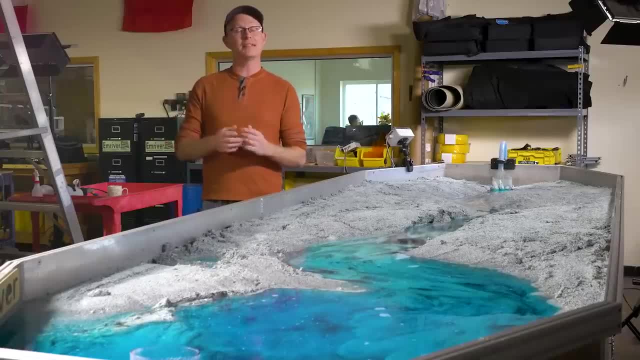 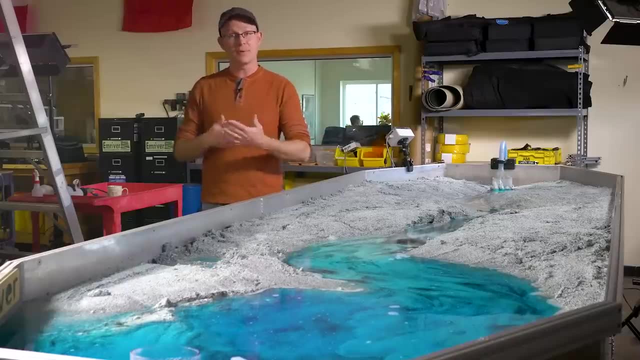 channels are usually short-term events, so the scale naturally balances itself once the river returns to normal conditions. But consider something longer term, like a changing climate, where a river is receiving more and more or less and less flows year over year- In this case, lanes'. 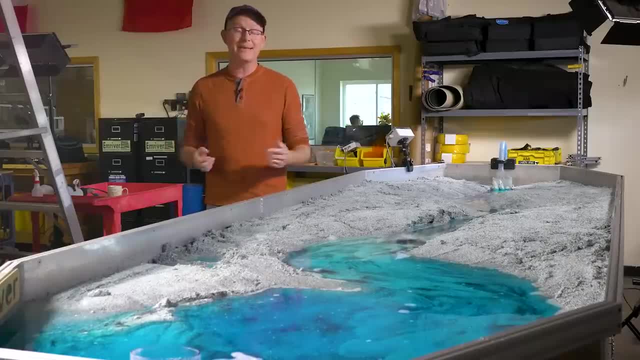 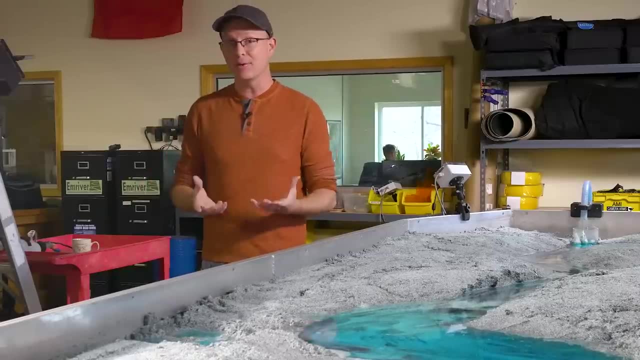 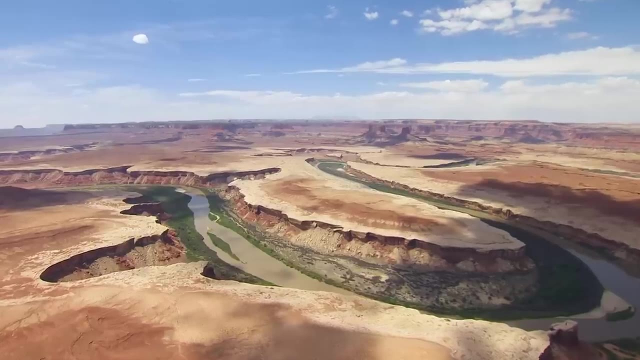 balance will shift toward deposition or erosion and stay there. But a central part of Lane's theory is that over time, factors will naturally adjust themselves to bring the river back into equilibrium, And that happens mostly as a result of the fourth parameter that we haven't discussed yet: the slope Erosion. and 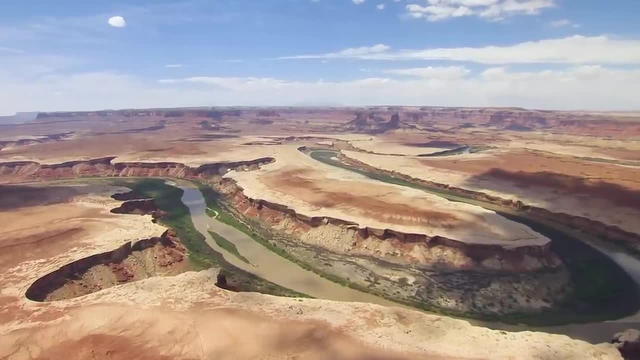 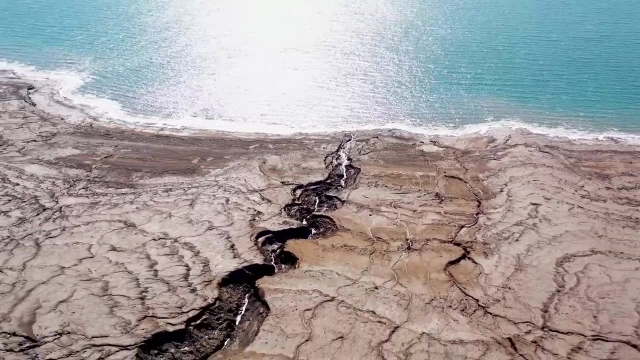 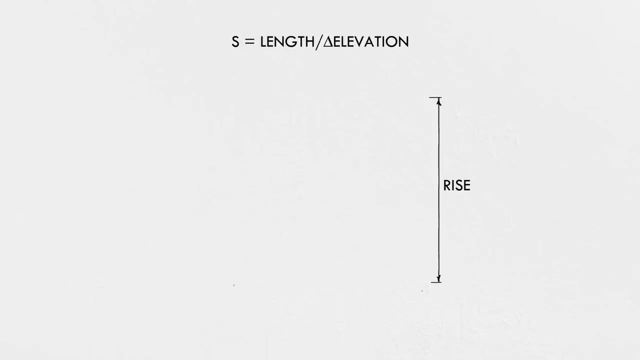 deposition have a natural feedback mechanism with the slope of a river. But how can a river change its slope? After all, the starting and ending points are relatively fixed. Slope is defined as the length of the line divided by its change in elevation, The rise over the run, if you remember from algebra, class A. 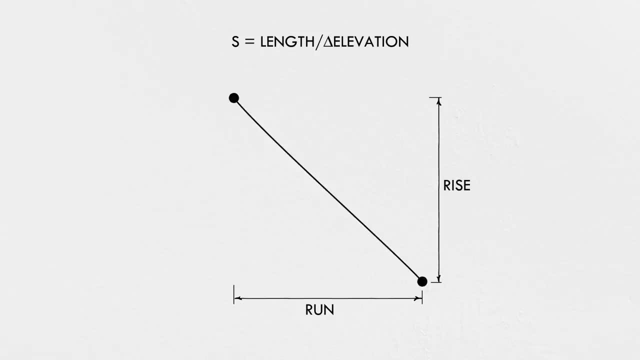 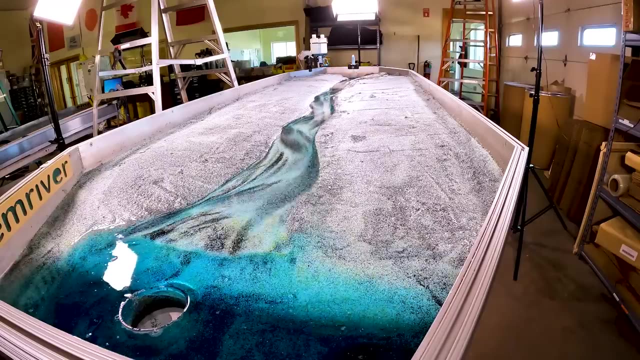 river really can't change the rise or fall between its source and mouth, but it can change the run, its length. Consider the original example I gave you at the beginning of this video. Its lane balance was all out of whack: Too much water and. 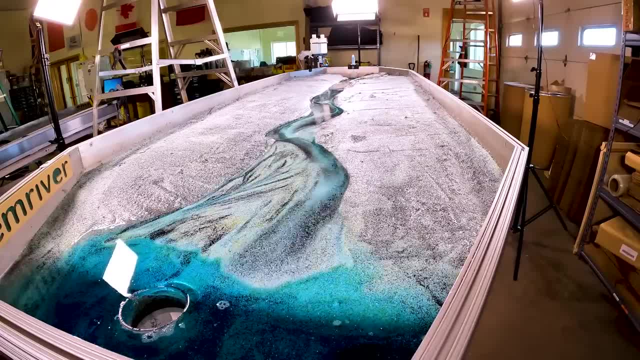 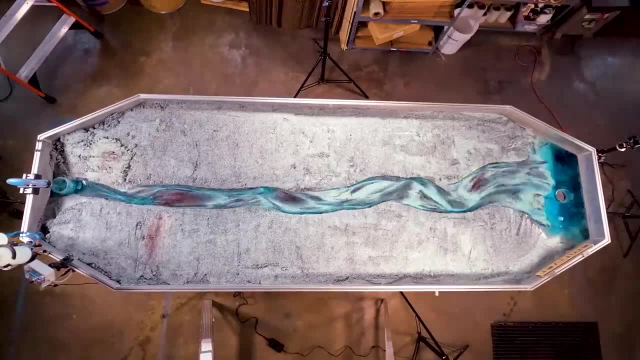 too much slope created a situation where it eroded out significantly at first, but over time it started to change, And that's what we're going to talk about today. Over the course of a few hours, a new pattern started to emerge. The river started to meander. 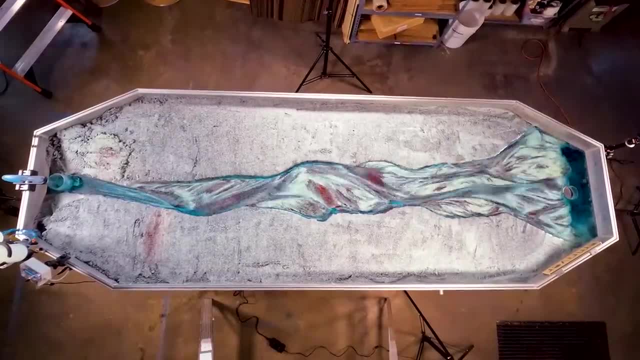 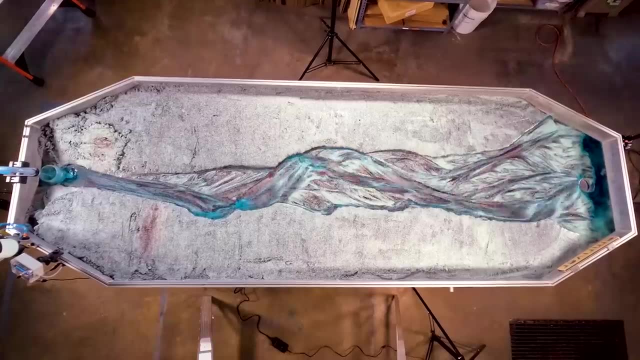 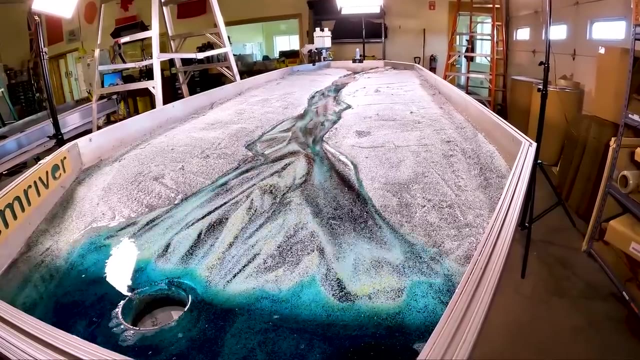 to lengthen itself by curving back and forth, creating a sinuous path from start to finish. That lengthening led to a reduction in the river's slope, naturally bringing the channel back closer to its equilibrium condition. But look closely and you'll still see sediment moving. It erodes. 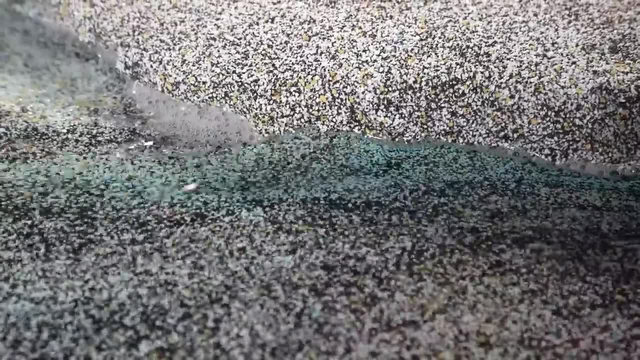 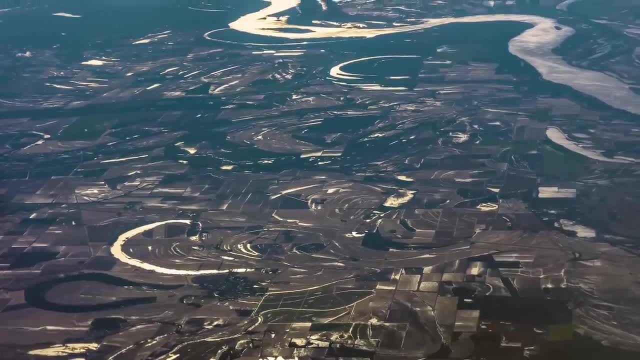 from the outside of bends where flow is most swift, called cut banks, and it deposits on the inside of bends where flow is slower, called point bars. This creates natural meandering of rivers and geographic features like oxbow lakes, where a river cuts itself off at a bend, leaving 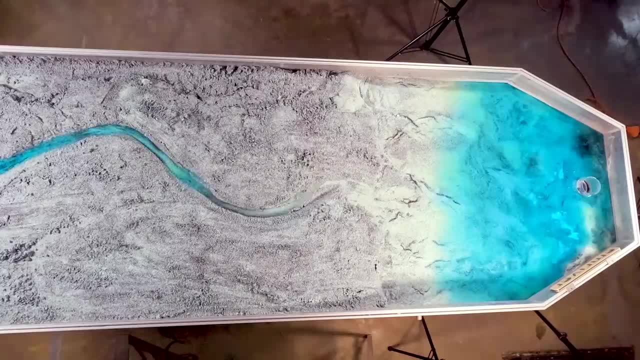 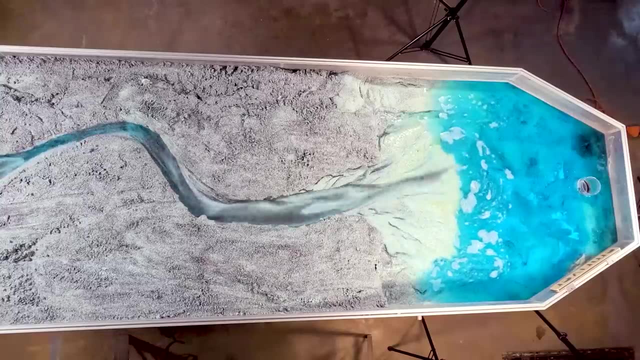 a curved depression behind You also see natural aggradation, where a river discharges into an ocean or lake, where sediment falls out of suspension, called a delta. These phenomena happen for most rivers and streams, even those that are quote-unquote balanced according to Lane's theory. 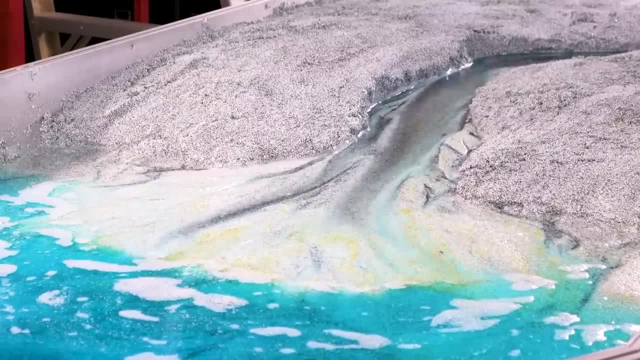 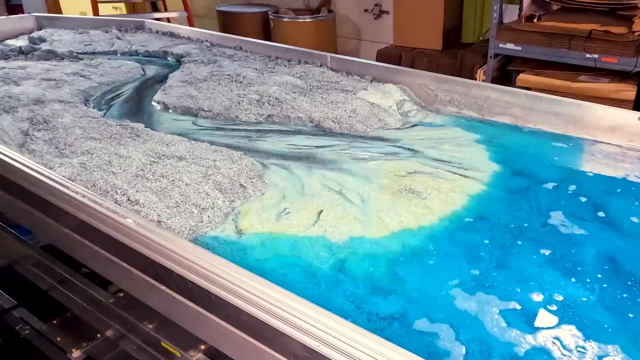 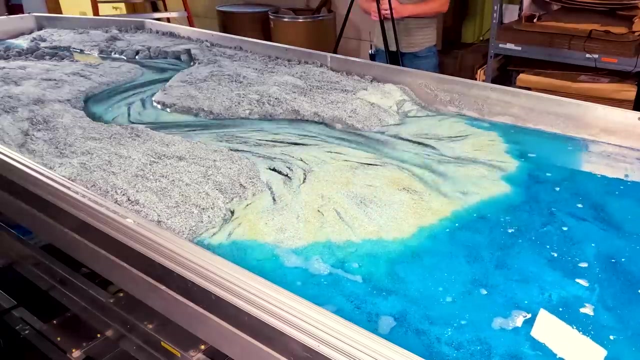 In reality, there's no such thing as a static state for a river. All the variables are changing over time. Floods, droughts, fires, debris jams, animal activity and many other natural processes ping the balance this way and that, and we haven't even mentioned the human activities that affect rivers at all. That's the. 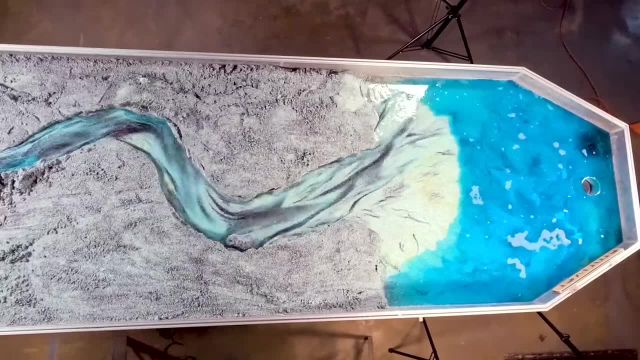 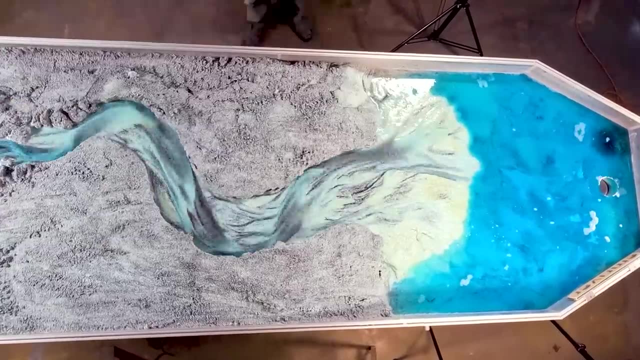 topic for the next video in this series, by the way, so make sure you subscribe so you don't miss it. In addition to the constant shifting of flow and sediment load, the natural processes that pull a river toward equilibrium are not very good. If you're interested in learning more about the 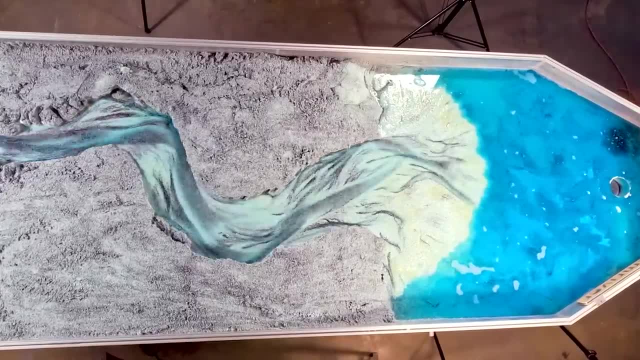 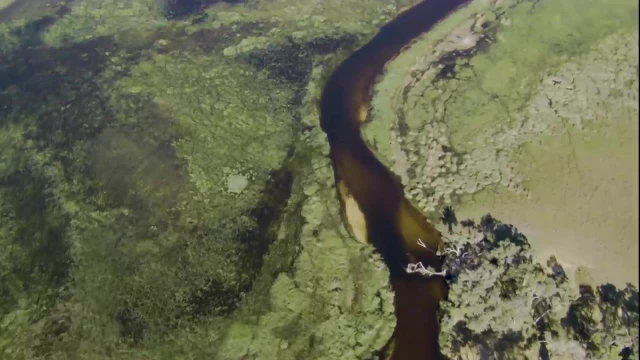 natural processes that pull a river toward equilibrium. be sure to subscribe to our YouTube channel. In reality, Lane's scale is always in motion, bouncing between erosion and deposition states at every point along a river or stream. We call this a dynamic equilibrium because, even when all 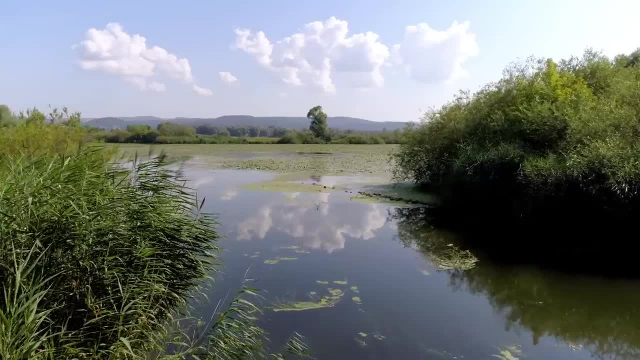 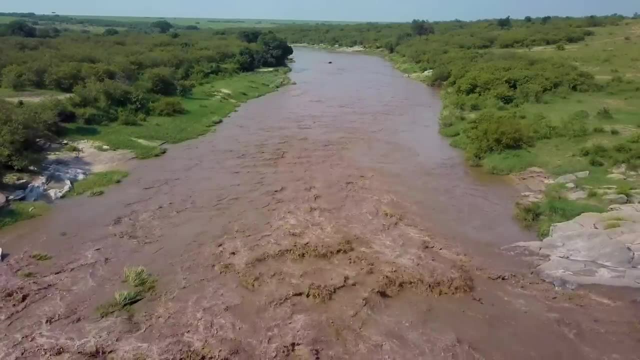 the factors of sediment transport are in balance. rivers still shift and meander. In that way, Lane's equation is more a way to characterize the magnitude of change than a binary measure of whether a stream channel is in balance or not. If you're interested in learning more about the 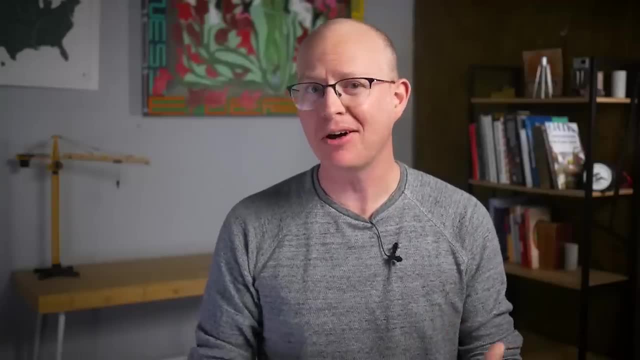 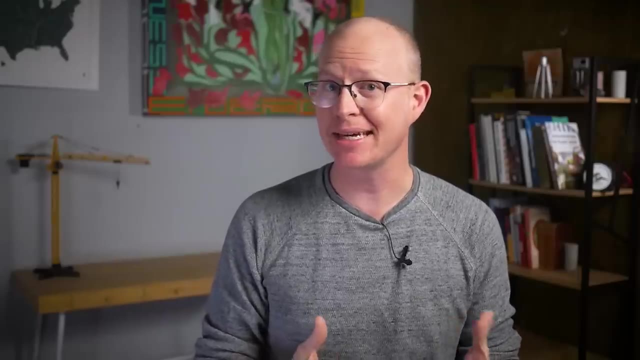 natural processes that pull a river toward equilibrium. be sure to subscribe to our YouTube channel And of course it's a simplification. I've been calling it an equation, but there's no equal sign to be found. It's really just a qualitative relationship that can't tell you exactly how. 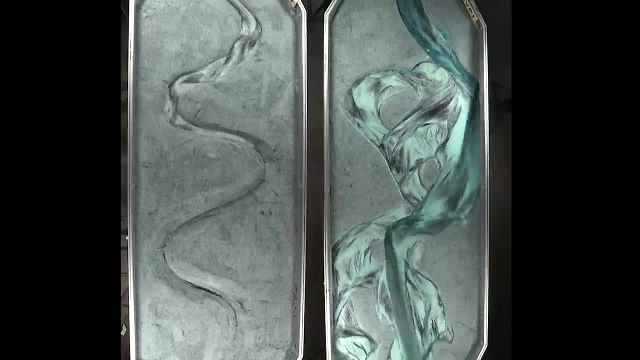 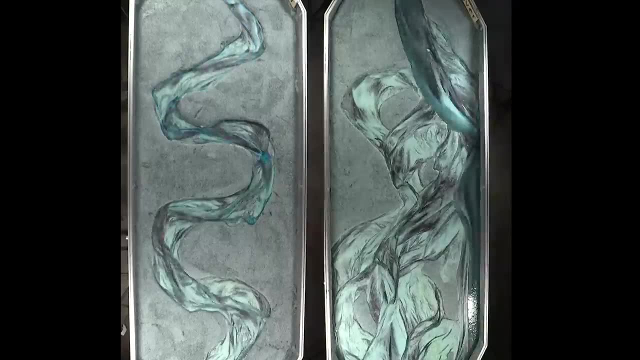 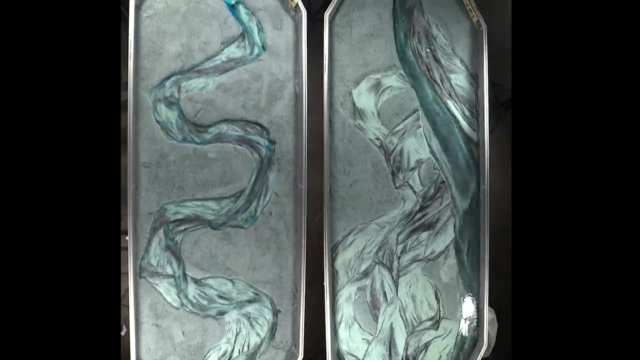 fast a river will meander or to what extent. There are also factors that it doesn't consider, like vegetation or pulsed flow, For example. imagine a scenario where the climate shifts toward more extreme periods of droughts and floods. Lane's relationship looks at averages. 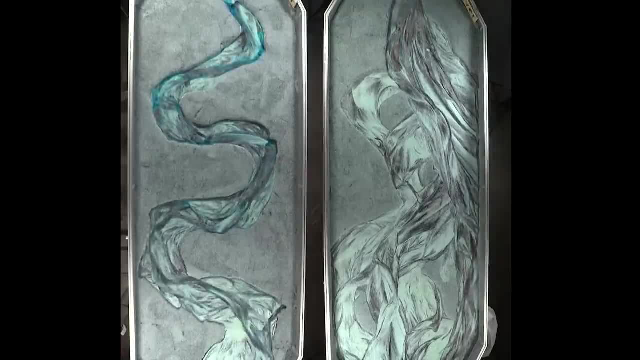 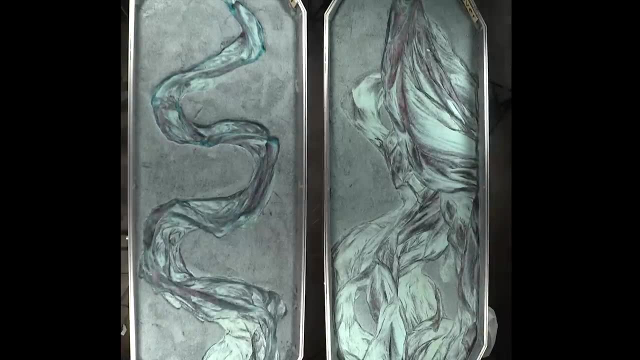 so if one river has a relatively constant flow, while an identical river has pulses of high and low flows, as long as their average flow is the same, Lane's relationship would assume they would behave identically. Well, we decided to try it out. See if you can see the difference. 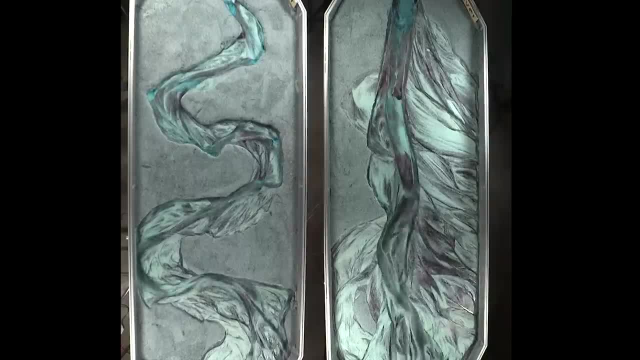 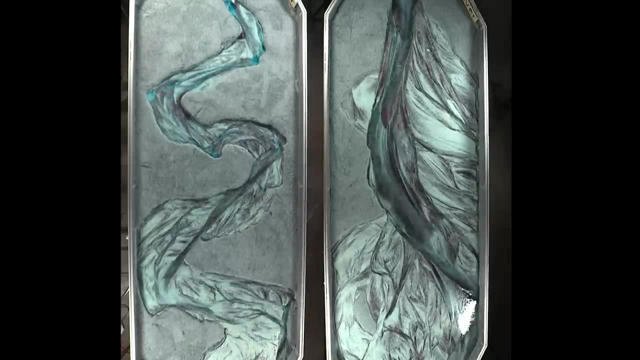 Even if Lane would predict similar behavior between the two models, it's easy to see that the pulsed flow model experiences much more erosion and faster movements of the channel. Clearly, we still have progress to make in our understanding of how rivers and streams behave. 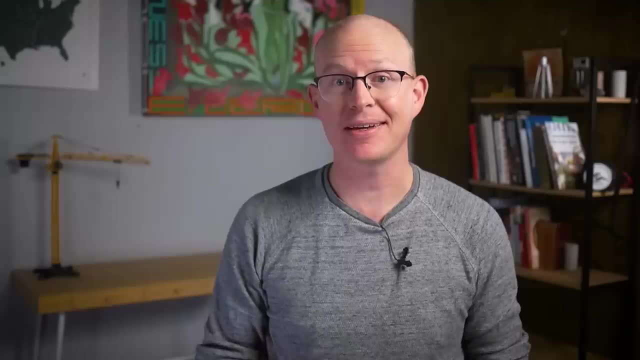 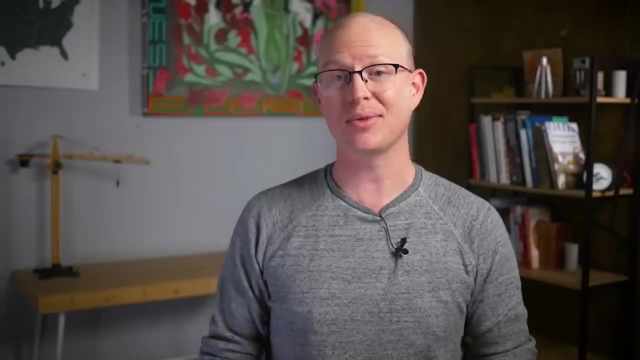 over time, under the wide variety of conditions that they face, From the tiniest urban drainage ditches to the mighty Mississippi. rivers and streams have enormous consequences for humans And, like pretty much everything else, the river can still move. So if you're looking at a river,